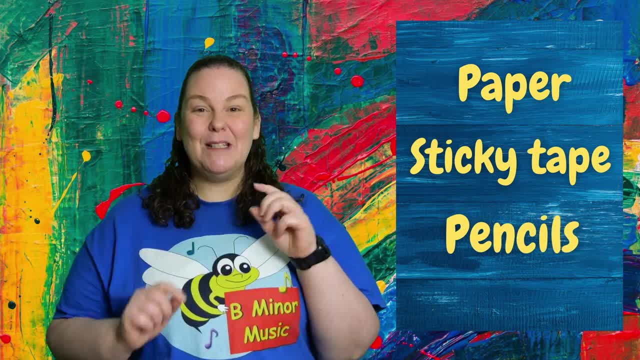 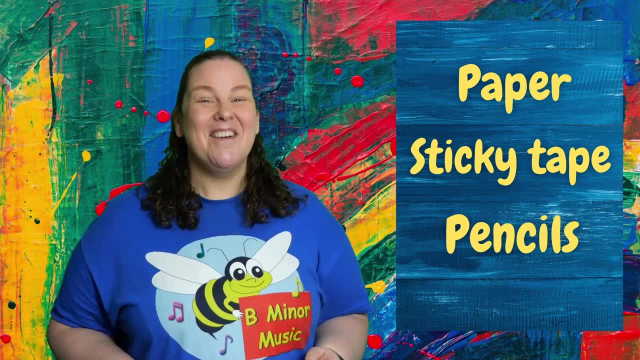 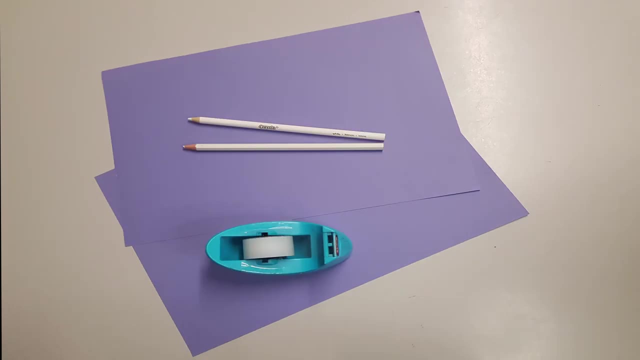 tape and pencils. Now what I'd like you to do is pause this video, grab those items and, when you've got them all, come back and press play and we'll make them together. Ready and go. I have some tapping sticks. do you have them too? 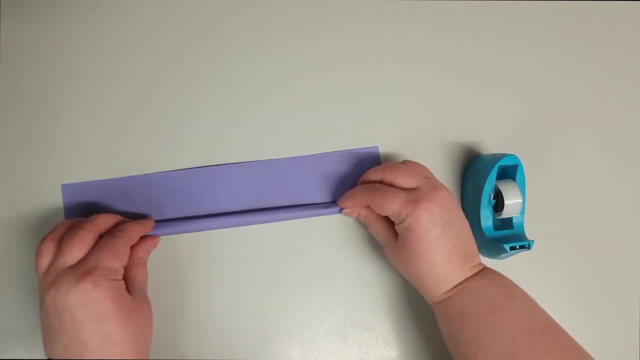 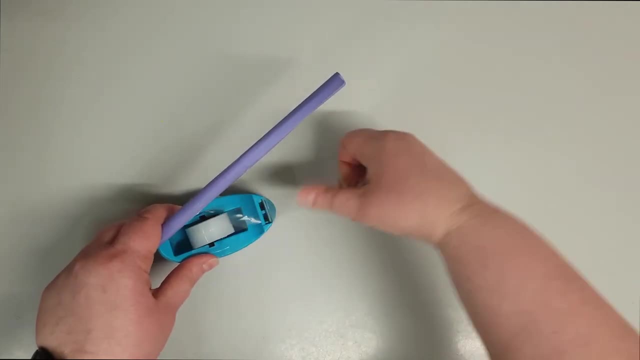 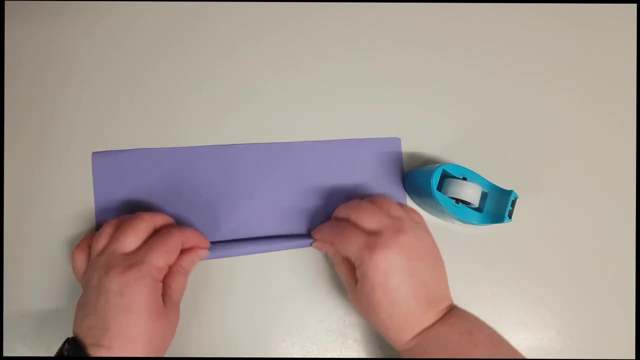 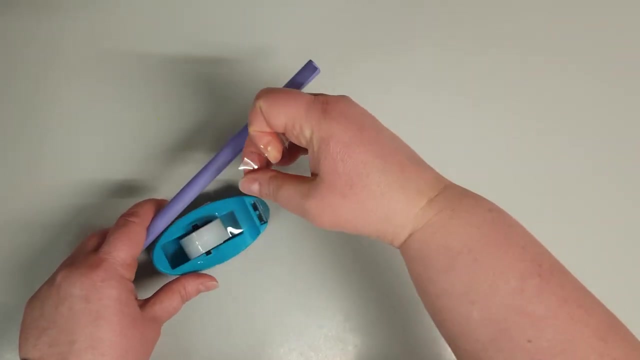 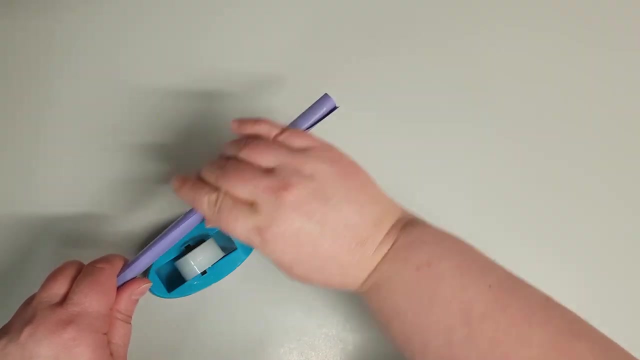 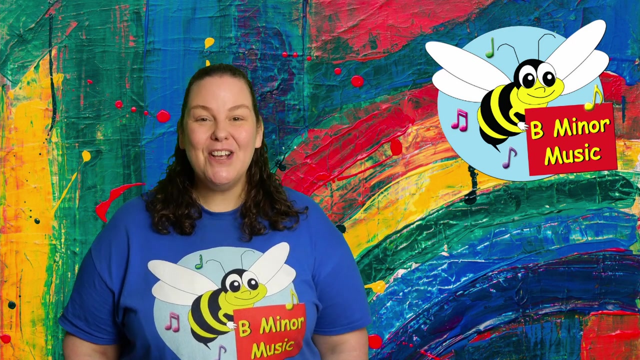 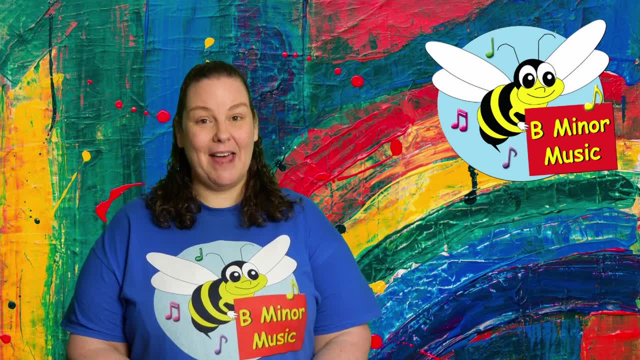 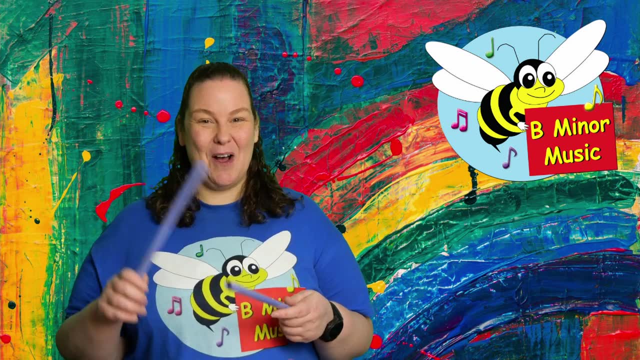 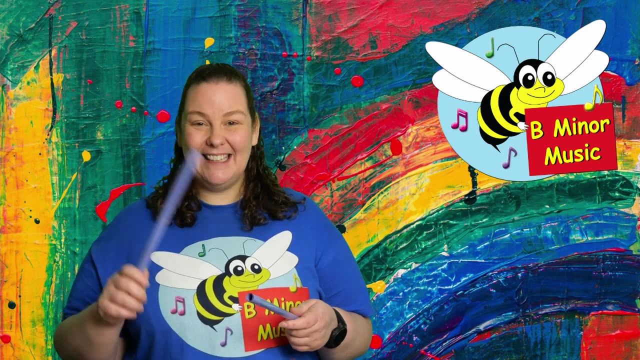 our tapping sticks today is a Torres Strait Island lullaby. It's a lullaby that's been passed down for generations and it's called Inanay. Can you tap your sticks together like this? Great job, Inanay kapuana. Inanay kapuana. 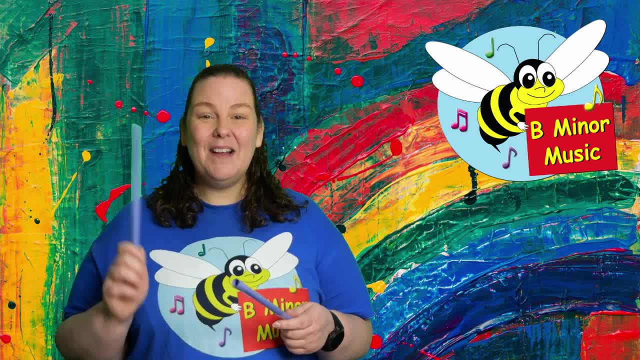 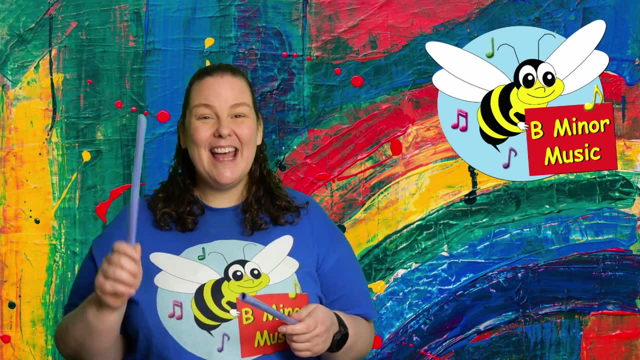 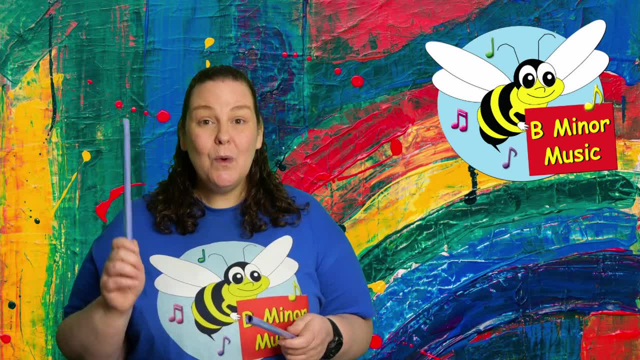 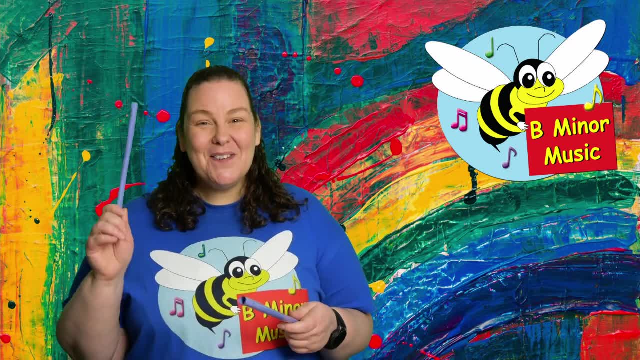 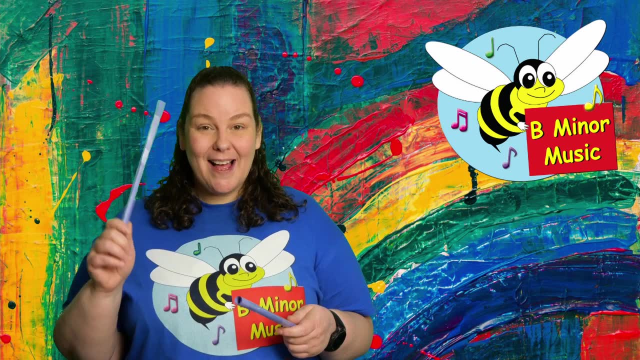 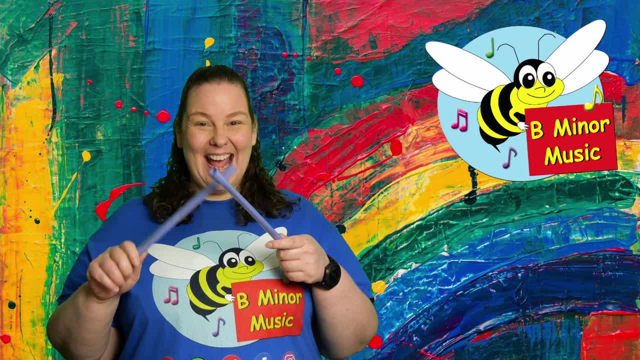 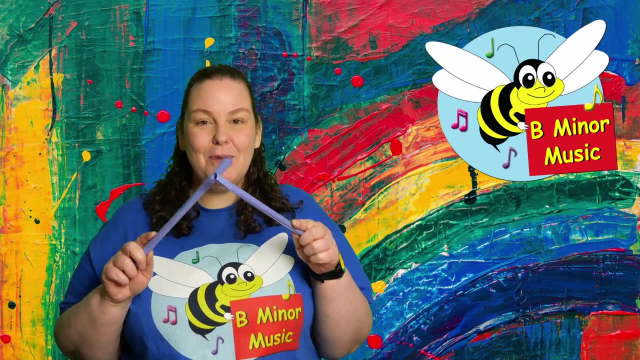 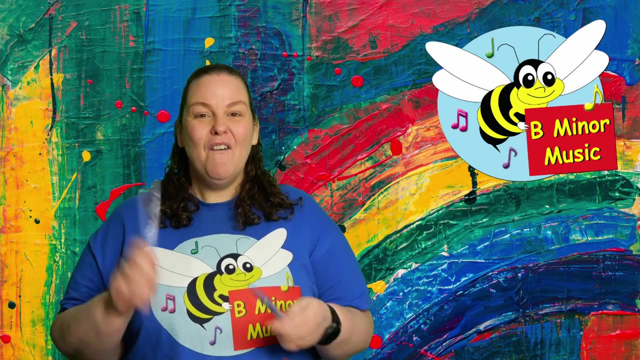 Well done. Give yourselves a tapping stick, clap, Hooray. All right, we're going to do some soft and loud now. So in music we call soft piano. So can you tap your sticks together, piano quietly. And then we're going to do loudly. Now, loudly, music is called forte. 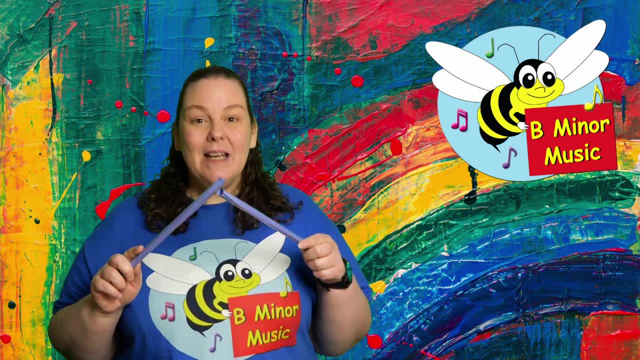 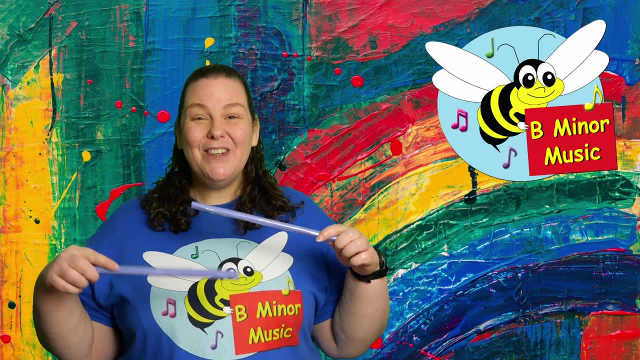 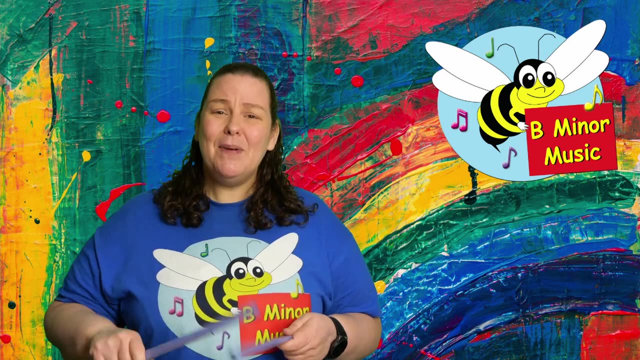 Let's start off by doing piano Topping, topping, piano top Topping, topping, just like that. Roll them over, roll them. so Now get ready, off we go, Topping topping, forte top Topping. 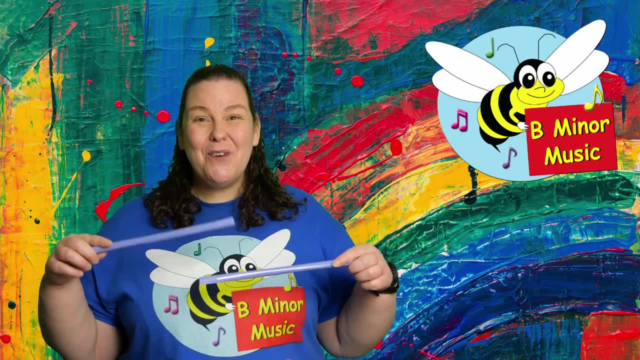 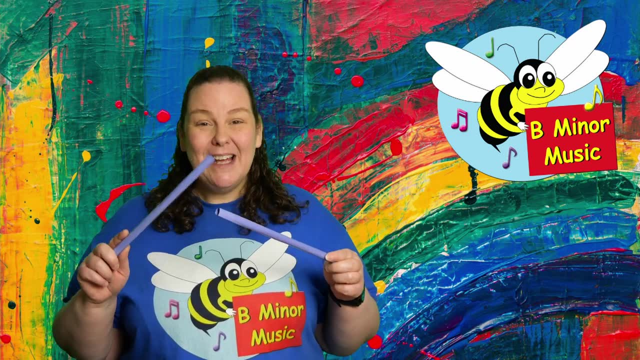 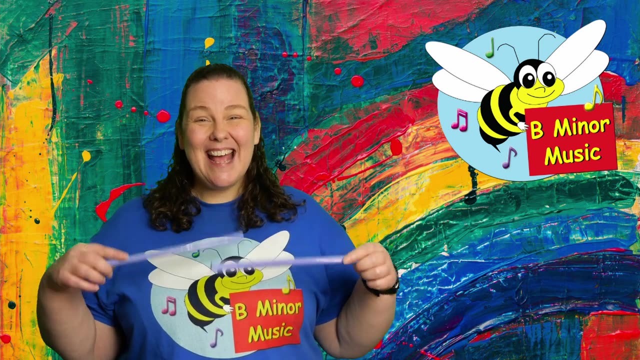 topping. just like that, Roll them over over. so Now get ready, off we go, Topping topping, piano top Topping topping. just like that. Roll them over over. so Now get ready, off we go Topping. 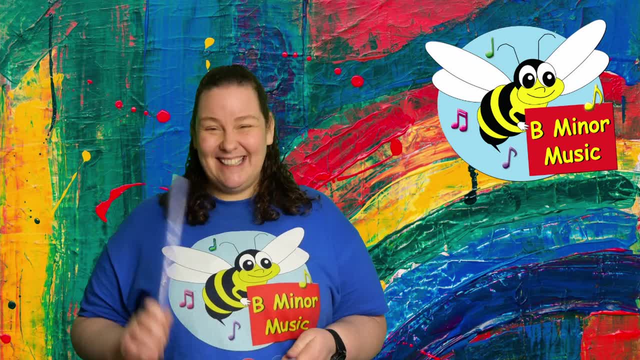 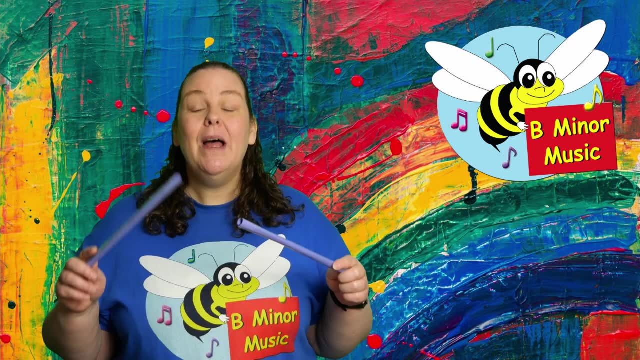 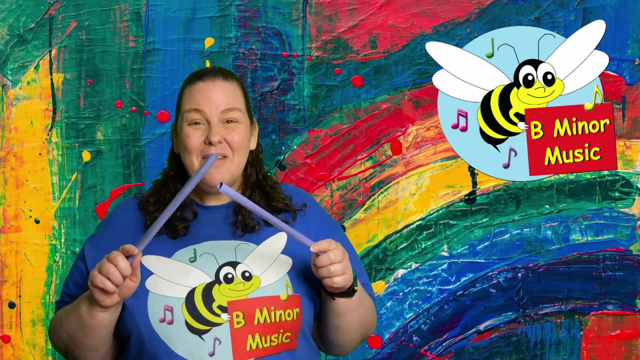 topping forte top Topping topping. just like that Roll them over over. so Now get ready, off we go. Topping topping piano top Topping topping forte top Topping. topping piano top Topping. 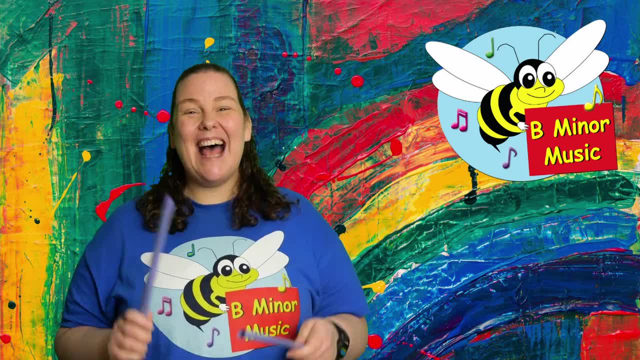 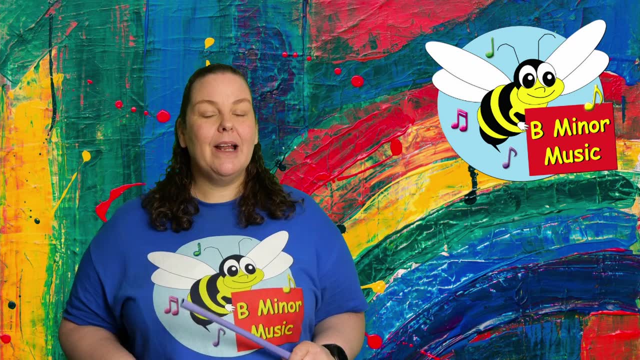 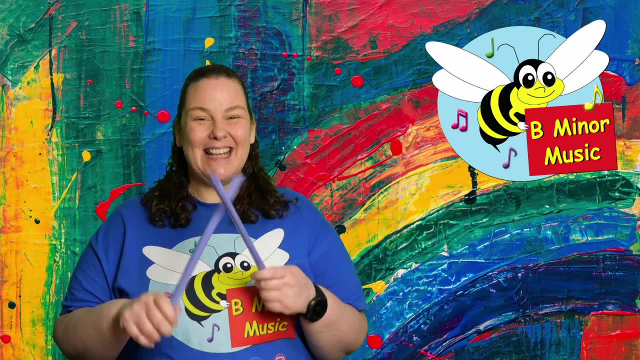 topping forte top. Well done. Give yourselves another tapping stick, clap. Fantastic. Now this one. we're going to use a different rhythm. We're going to clap our sticks together twice, Tap, tap, and then we're going to bang in front of us. Tap, tap, bang, Tap, tap, bang. That's it. 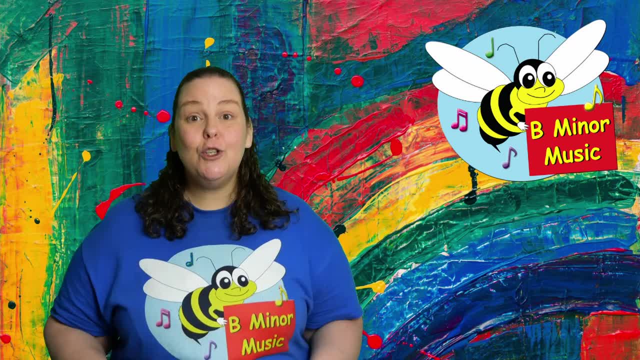 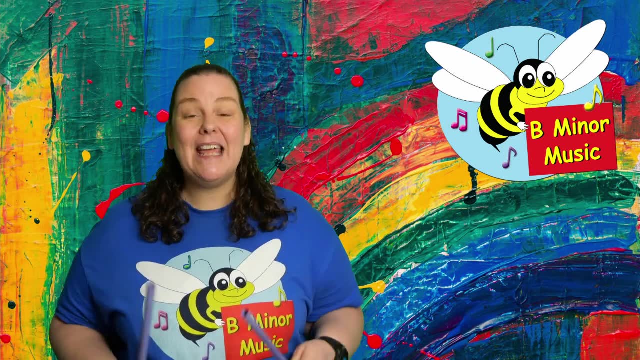 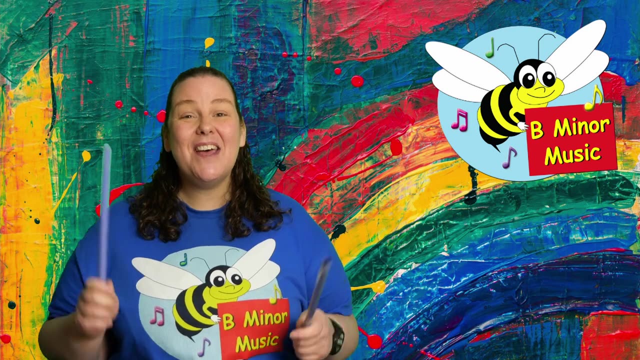 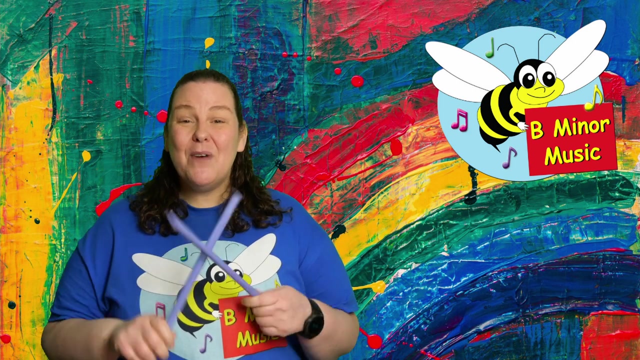 Oh, you're going to do it again. got great rhythm. Monday, Tuesday, Wednesday, Thursday, Friday, Saturday and Sunday- They're the days of the week, and night we sleep and during the day we dance and leap. Singing, we will, we will rock you. Singing, we will, we will rock you.